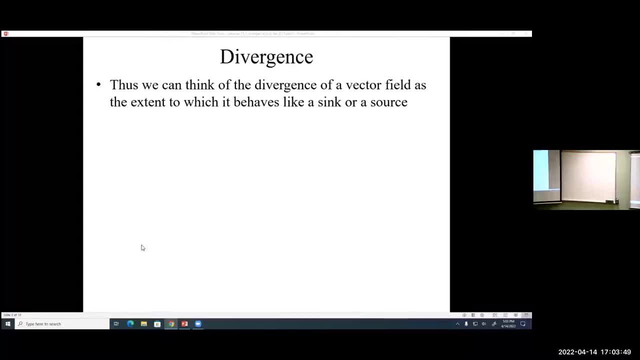 You know it's not an absolute, It's not like gravity, where it's all going towards the point, Or, you know, it's all going away from the point. It could be, but it could be just some is going towards it and some is going away, or vice versa. 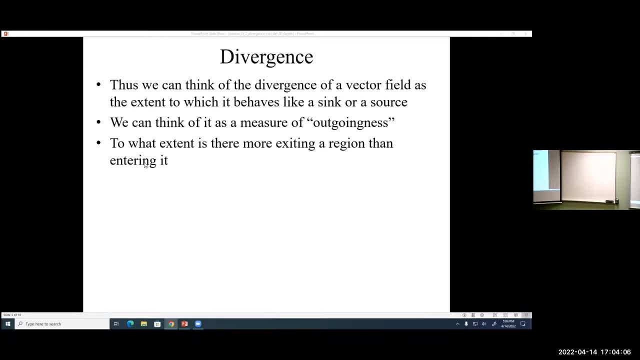 So think of it as like a measurement of outgoingness. The nice thing about divergence is, you know we'll do it at a point today, but later this semester we'll be able to use divergence to measure flux or the amount of something going on. 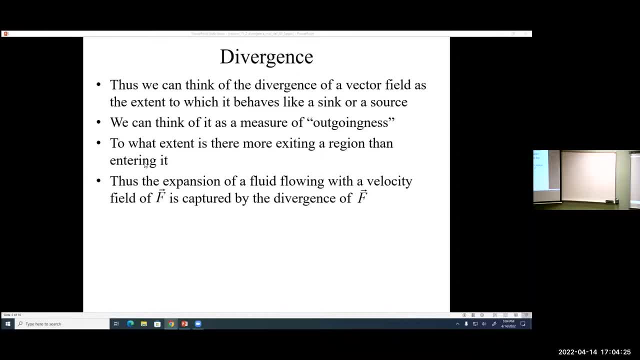 And we'll be able to measure it out or in on an entire surface using an integral, Because an integral will add up all the points. What's that? Yep, we'll get our flux integrals in. So the expansion of a fluid with a velocity field f is captured by the divergence of f. 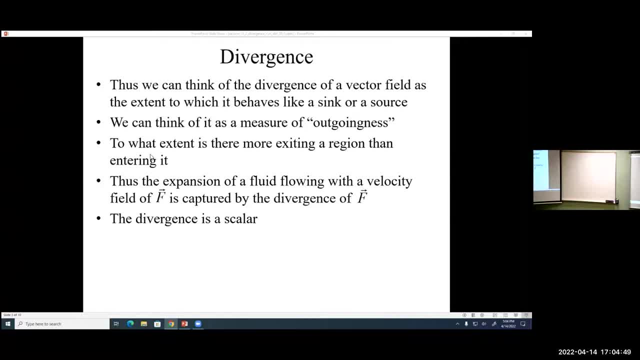 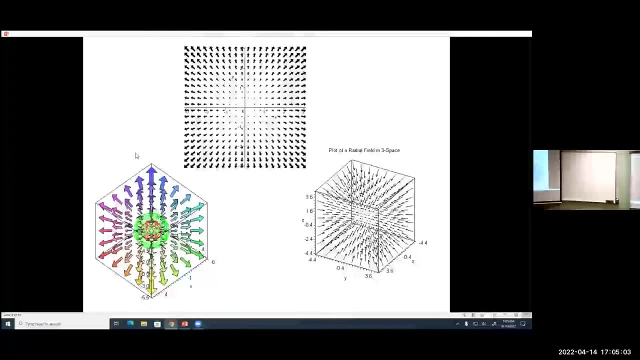 One thing I want to mention. divergence is a scalar. It is just a positive or negative number. Positive means it's acting as a source, Negative means it's acting as a sink. So here are, like, some really obvious examples, right? 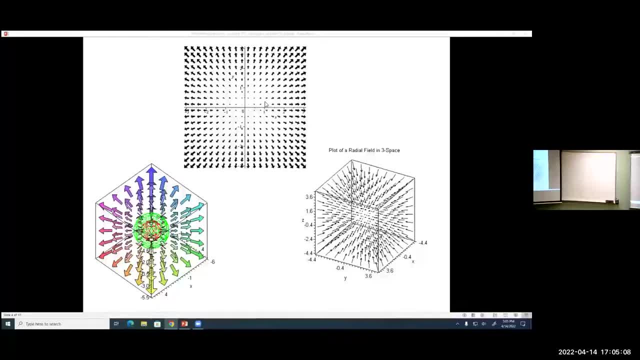 We can see that the origin is acting as a source. Excuse me, Thank you, In these two examples here we can see the origin is acting as a sink. So again, what, what diversions, what divergence does? is it basically measures the outgoingness or attractiveness? at any single point. 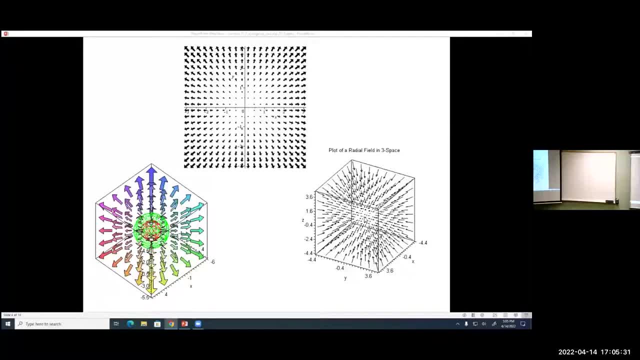 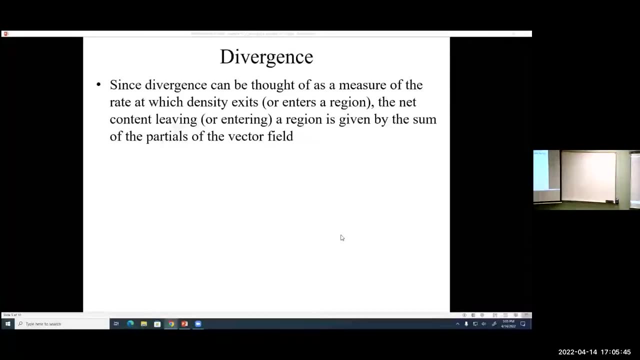 Not that any point is necessarily all repelling or all attracting, but it measures. is it more attracting or more repelling at any given point? All right. Well, how do we calculate it? This is the easy part. It comes from the partials. 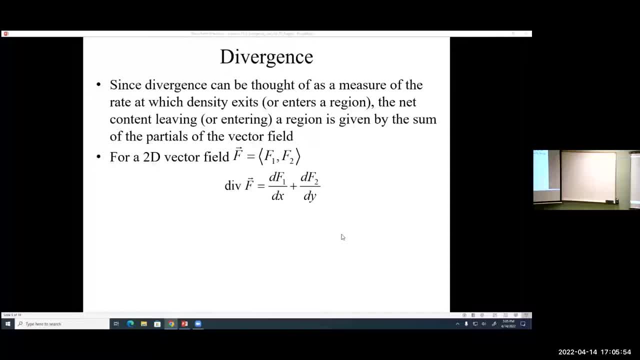 Because think about what we're doing. We're looking at the way something is changing, the way something's going towards it or away from it. So what we're going to look at are the partials. Are they positive or are they negative? 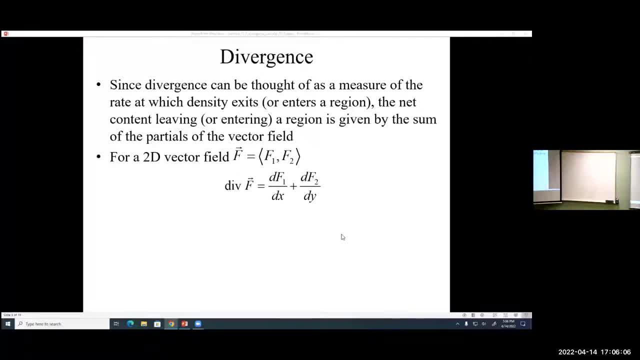 And we sum them together to get the total amount of divergence. So a 2D vector field. we sum up the partials And notice there's nothing crazy going on here, right? It's the partial of the partial, So the first component with respect to X, plus the partial of the second component with respect to Y. 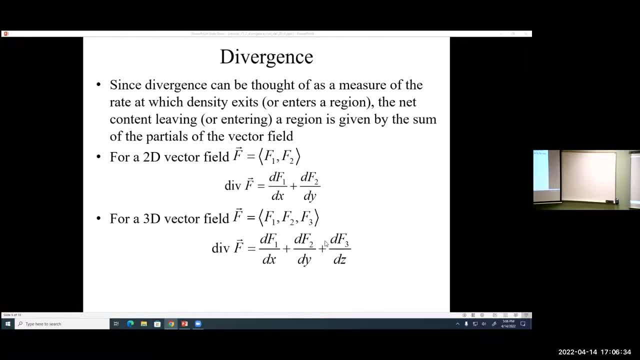 The 3D flux, we add on a third component. Now I'm pointing this out because you'll see, when we look at curl they actually flipped. So calculating divergence is it's like the gradient, almost. It's about as easy as anything we're going to do. 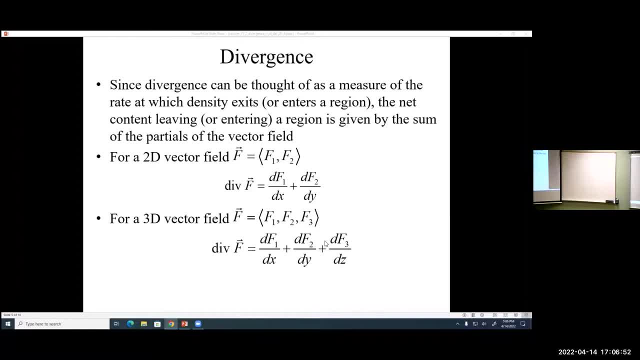 It's long Because we're very good at partials. now All we're doing is summing up the partials of each component And just remember that each component is lined up with your first component, X, second component, Y. third component, Z. 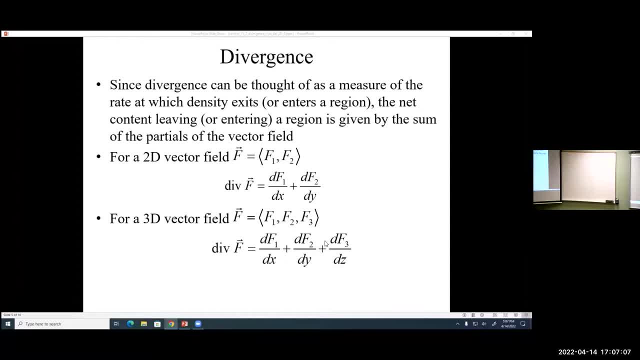 Now, obviously, you do not have to memorize this formula. You have the note card for the exams, or you can use a note card for working on the homework. We just need to know how to use it and have an idea of what it's telling us. 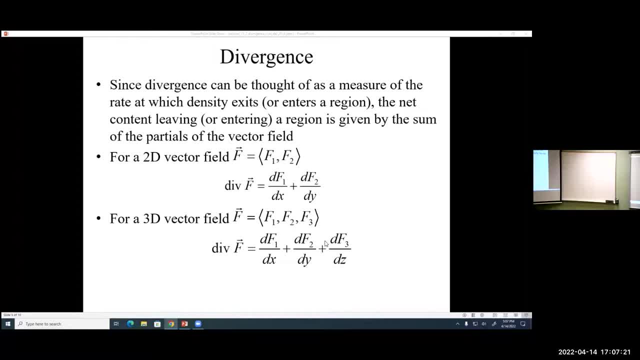 All right, One of the things I'll mention- And I have links And they weren't linked up to the calendar, So I put them into the calendar too. There's a website I like called Better Explain, that gives some intuitive explanations to some of the concepts in math. 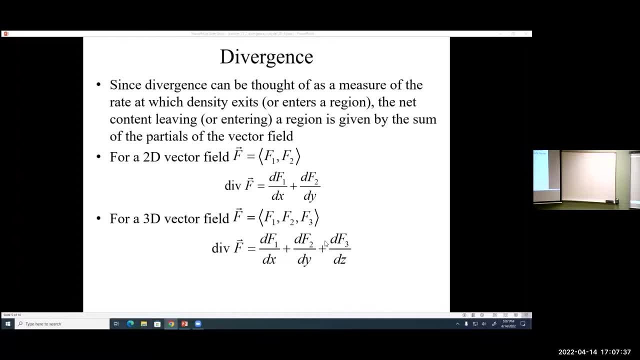 And so I linked its intuitive explanation for divergence and curl. So you know, if after our talk today, you're still, like you know, I'm not quite sure what I'm looking at with divergence or with curl, Go check out one of those links. 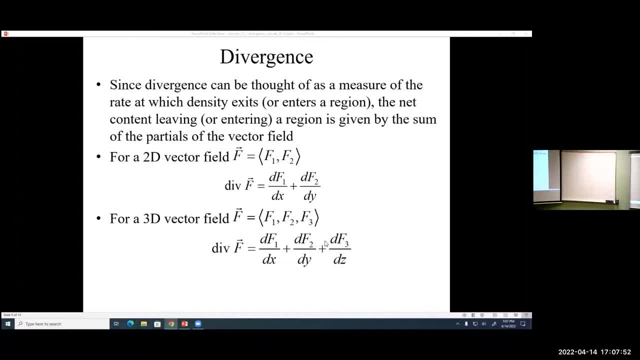 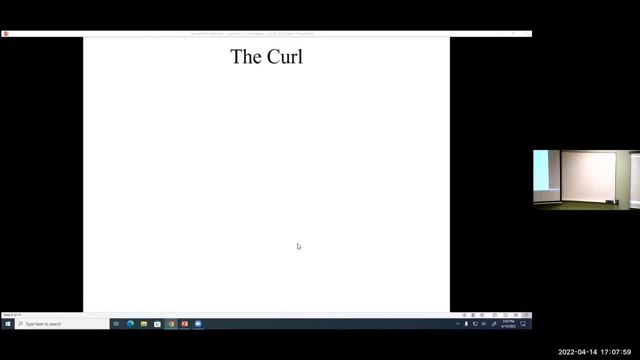 See what you think. I think they do a good job of kind of giving some real-world examples. Okay, Let's talk about the curl. So the curl calculates the amount of rotation of a vector field at any given point. So just, it's similar to divergence in that it calculates an attribute of a vector field at a single point. 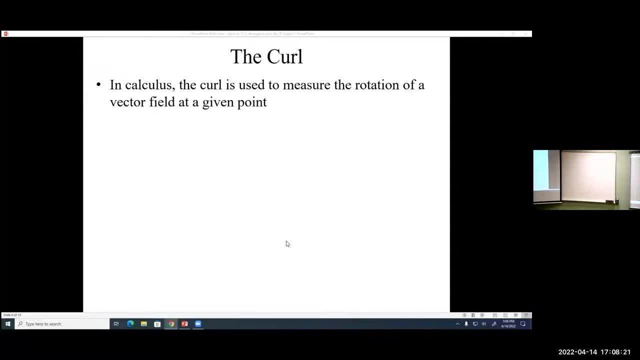 But the attribute it's looking at is different. Okay, Now we're looking at its tendency to rotate at any given point, And what we can do is we can add up the curl at all the points to get the circulation of the vector field. 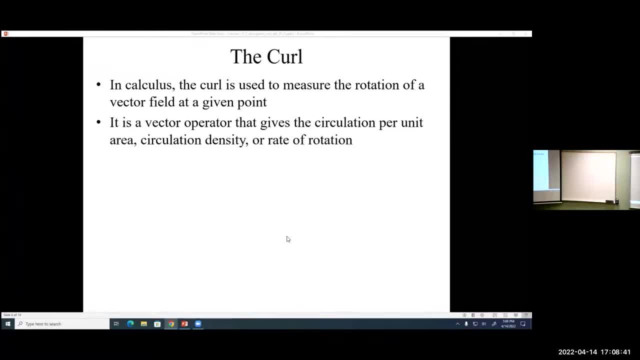 So the curl is actually a vector that gives what we call the circulation density or the rate of circulation. Again, you add that up, You get the total circulation, because we're accumulating rate. So if you imagine taking a whirlpool and then you shrink it down smaller and smaller, while keeping the force the same, 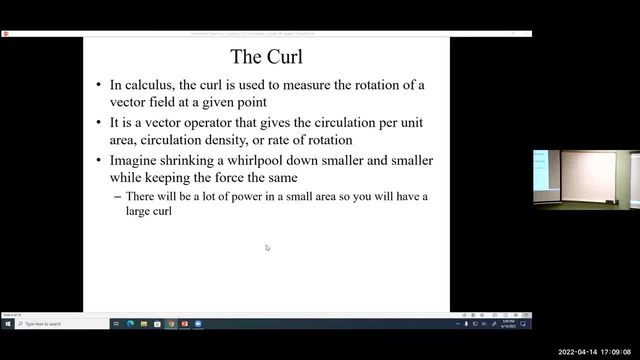 there's going to be a large amount of power all of a sudden in a small area, So we would get a large curl. The faster that rotation is, The slower the rotation, the smaller the curl. Okay, So again, it's a measurement of rotation. 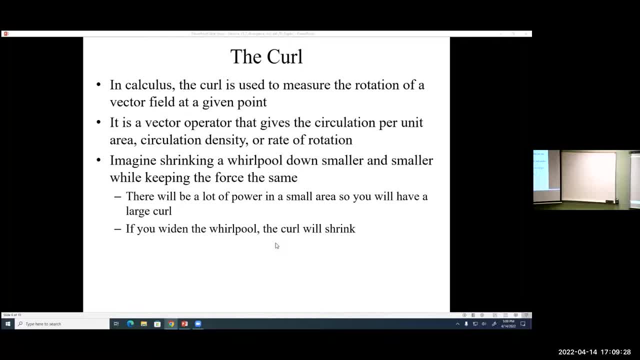 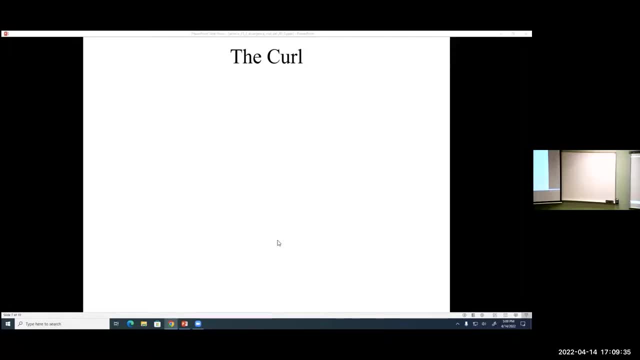 We can have a zero curl, which we're also going to talk about here in a little bit, because that makes something very interesting for us too. When we give you kind of an idea of what this curl is. What's that? Well, it kind of I see where you're going with it with, like, if we think of a sink and a drain going down. 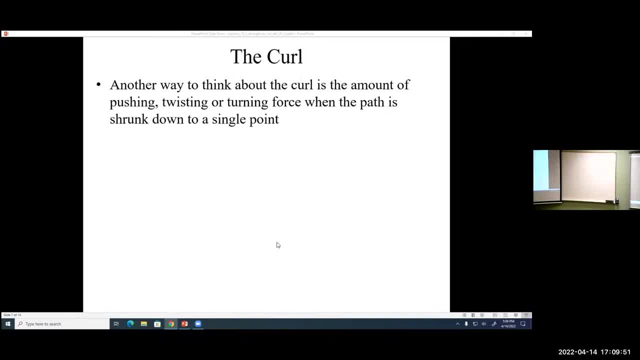 But there I want to be careful of Using it with a sink, because they are a little bit different. right A sink is, it would be an attractive force, Whereas curls, a rotational force, doesn't necessarily go down, It doesn't. it doesn't necessarily pull things towards it. 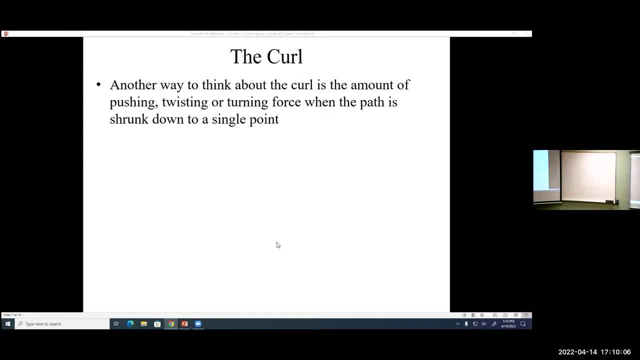 It spins things around. So the curl is the amount of twisting going on when the path is shrunk down to a single point. So you know, imagine putting like a flat surface in water, like that site better explain talks about using an ore. 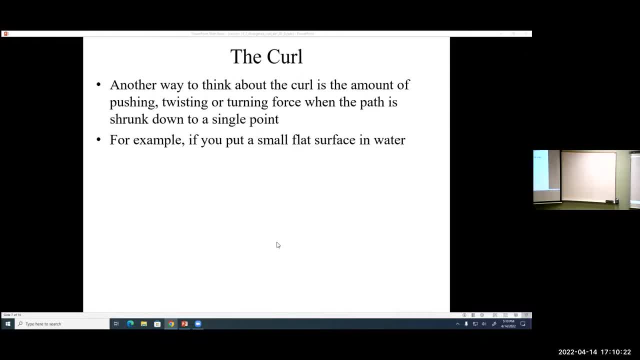 Right, imagine putting an ore down in the water. Okay, what happens with the ore? Does it go forward, Does it go back, Or do you feel it twist? If you feel it twist, that would be the curl, That would be a circulation density, because what's happening is one side is getting pushed harder than the other. 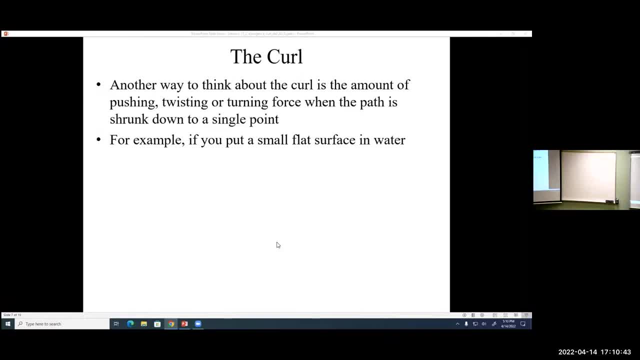 It's not an equilibrium. When it's an equilibrium, we have a zero curl. The harder twist, the larger the curl. no twist, We got a zero curl. Now here's. this is going to be something that's going to be really interesting for us as we go on, because we're going to start to talk about conservative and non-conservative vector fields. 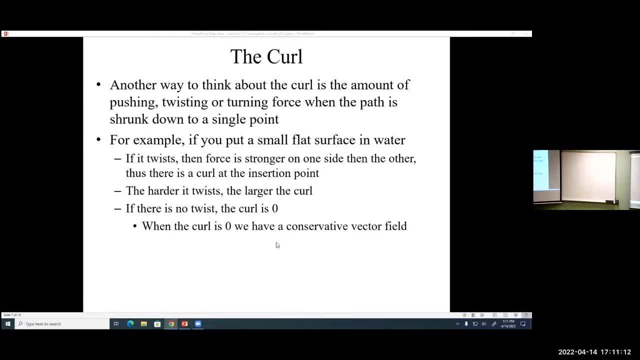 When the curl is zero. think of curl being zero as things being in equilibrium. We have what's called a conservative vector field, Which means it's path independent. In other words, no matter what path we take between two points through the vector field, the amount of work done by the vector field is going to be the same. 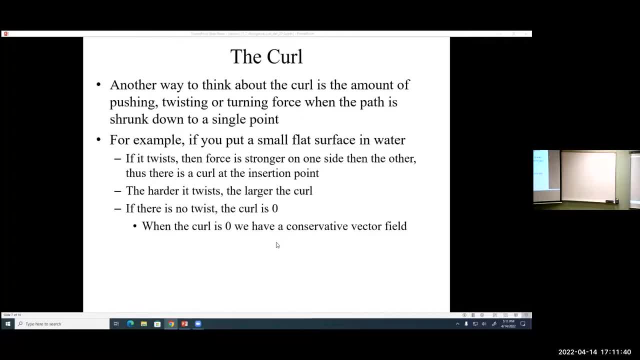 It's like what? Yeah, Yeah, we will relate it to some work stuff here, Not today, That's. you know, we haven't talked about line integrals yet. That's where we're going to go to on Tuesday And all of a sudden, this idea of conservative vector fields is going to be really important. 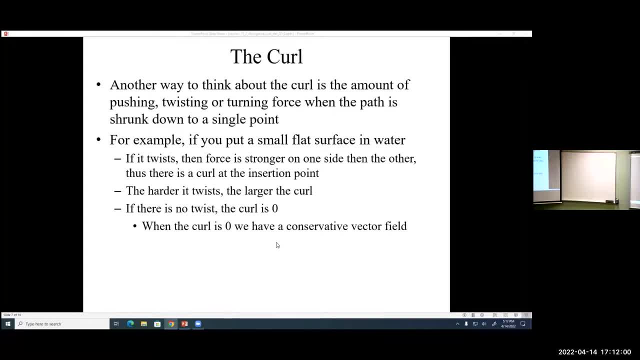 So we're going to start talking about it now. Well, now we already have a way of identifying it. If we get a zero curl- and it has to be zero for all the points- we get a conservative vector field, which means it's path independent. 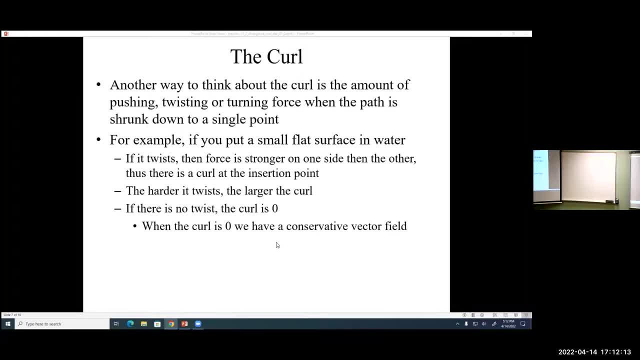 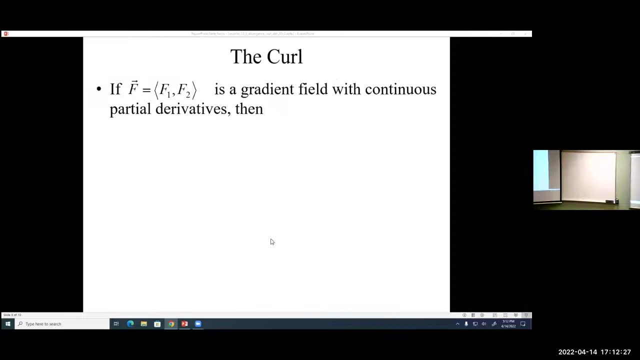 We're going to rehash all these terms again next week, So I don't want you to worry that. you know I'm throwing too much at you at once. It's going to come back again. Okay, Now let's assume that we have a gradient field. 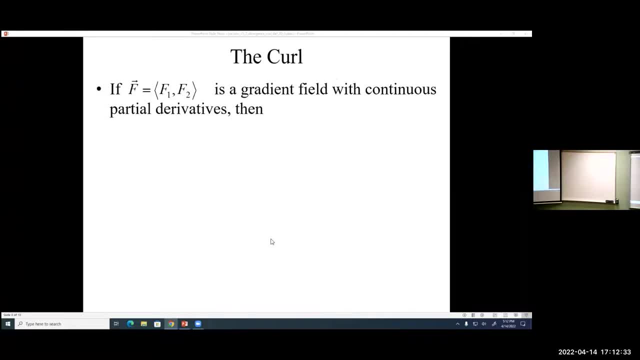 All right, we looked at this. We talked about this last time. A gradient field is a vector field, but not all vector fields are gradient fields. We have a gradient field if there is a potential function whose gradient made our vector field right. 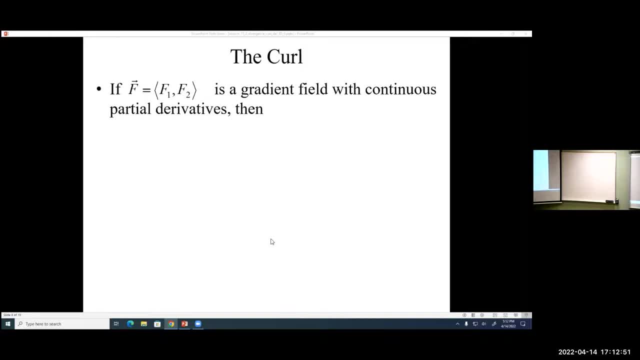 So if we know something's a gradient field, then we know it's made up of the partials of some function, Then we can calculate the curl df2 dx. So this is one where I said it's opposite right: df2 dx minus df1 dy. 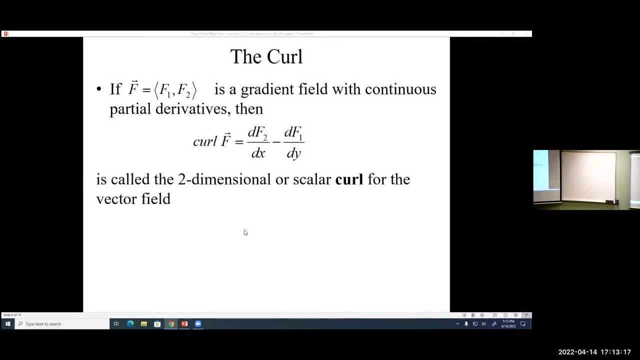 That's our 2D curl And we'll talk more again about gradient fields and potential functions next week as well, Because again, there's a lot of really cool properties when we know something is a gradient field that don't exist for all vector fields. 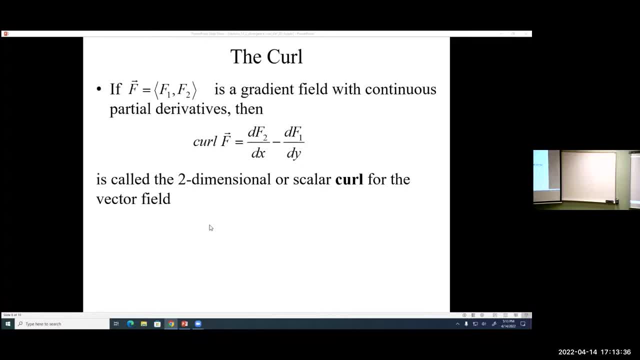 But if this curl comes out to be zero, the one thing we do know is we have a conservative vector field. Now think about what happens if we have a gradient field. Now, if we have a gradient field. So this would be the partial with respect to x. 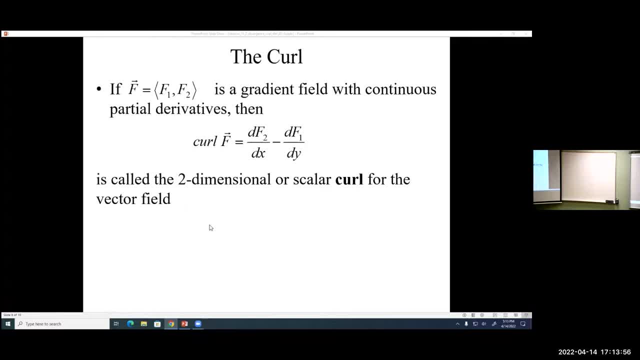 This would be the partial with respect to y. We'll talk about more about this next week, So I don't want to actually do it on here. So this is. this will be the partial. partial with respect to x. this will be the partial with respect to y. 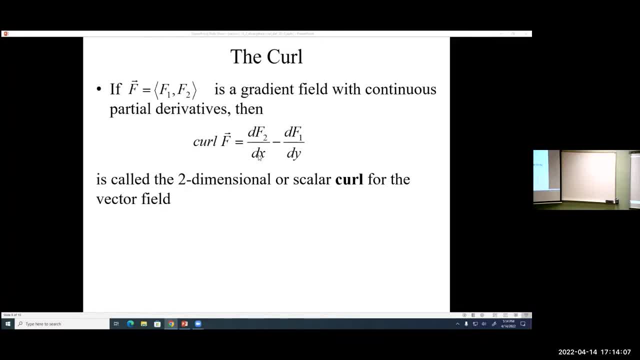 That means we would do the partial with respect to y, then the partial with respect to x. So this basically would be f sub yx. This here would be f sub xy. What do we know about f sub yx and f sub xy? 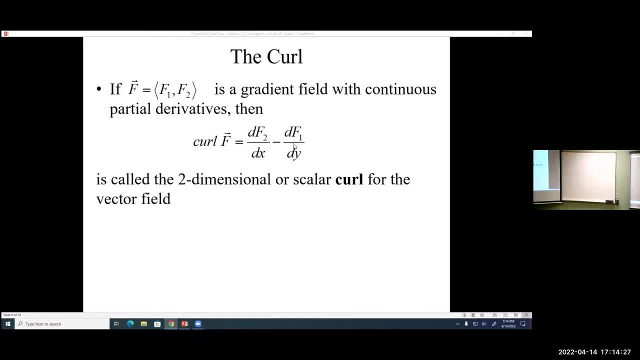 If we did everything right, they should be the same, which means we'd get a curl of zero. So all gradient fields are conservative. I kinda that was something we're gonna get into next week more explicitly, so I gave away the punchline. 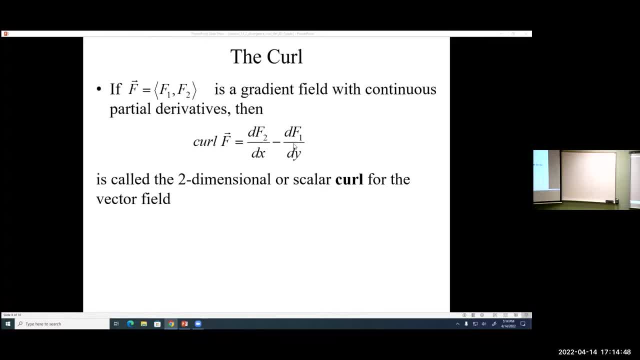 but we're talking about it now. so might as well, But we'll look at that more next week. Today we're specifically gonna look at calculating divergence and curl and using the curl to identify if we have a conservative or non-conservative vector. 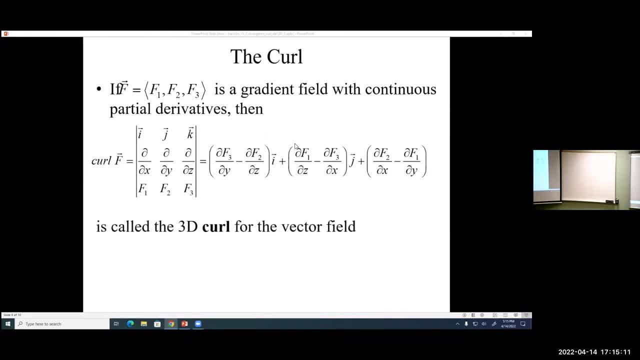 The curl in 3D. this looks kind of familiar right? This looks a lot like cross-product- Very similar, it's same idea as cross-product. So the curl in 3D of a vector field could be done as a determinant of a three by three matrix. 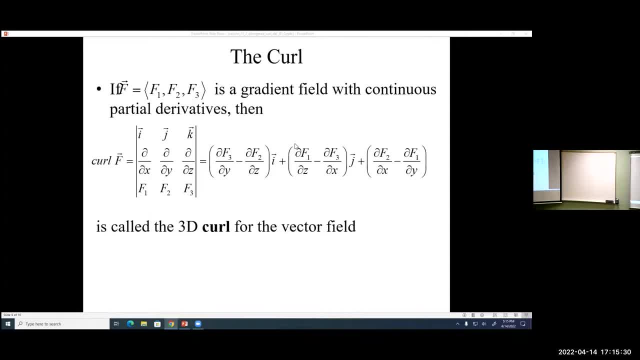 or you could just use this formula here. That's totally fine. You're gonna have your note cards. You can use Wolfram Alpha and say: find the curl of this vector field. That's fine too. One of the things I wanna point out here. 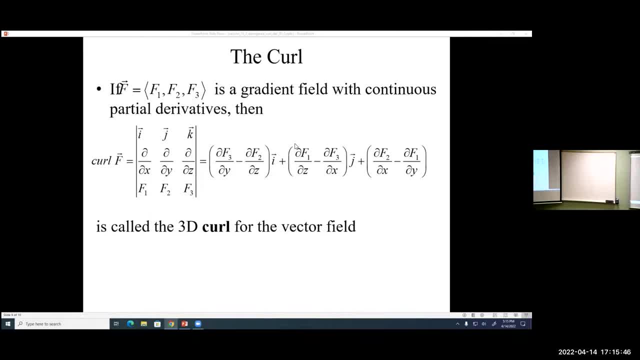 notice: the curl. Curl actually comes out to be a vector Right in 3D. So that means it has magnitude and direction. So the magnitude is basically the speed of rotation- nothing crazy going on there. but that means it also has direction. 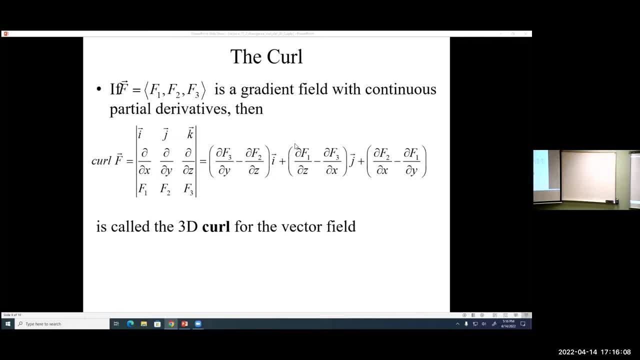 The direction. remember that, or example that we were talking about, The direction would be the stem of the or. okay, OK, so it's the axis of rotation. So let me do this so it's on camera. So if the direction you're, if the curl goes. 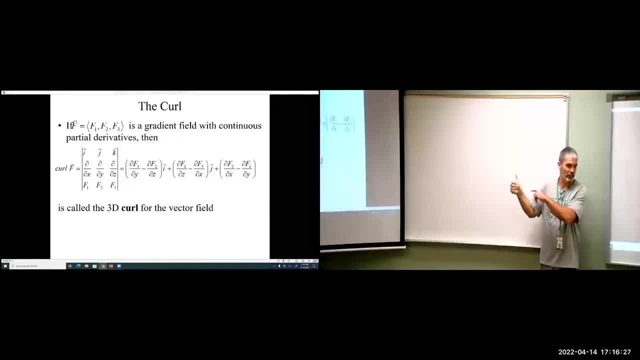 in the direction of my fingers. the direction the vector is pointing is upwards, in the direction of my thumb. If it was curling this way downwards- As you can imagine, because we're in 3D- we could have a curl that goes like this right: 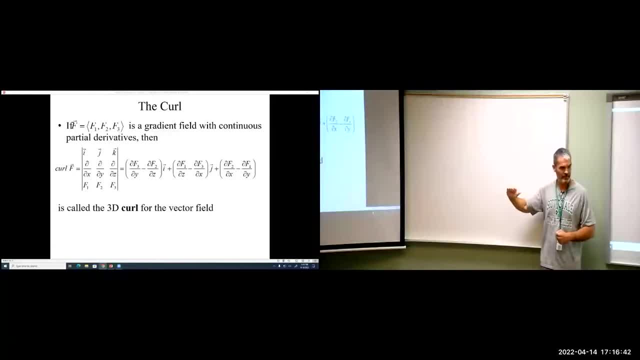 Any possible direction, and what the vector direction gives us would be that piece of the ore that we're holding in the water. It's like rotational rotation around the axis. Exactly, it's that rotational axis. That is not going to be a big deal for us. 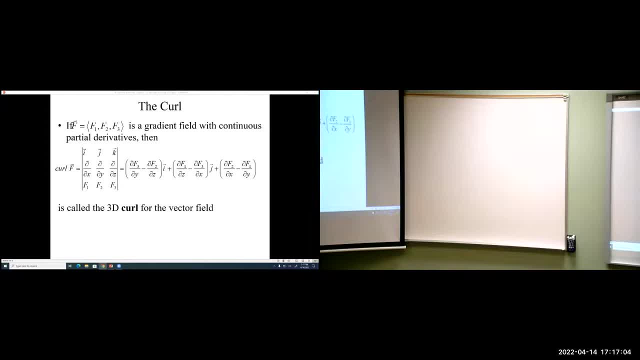 because we don't really use that direction very much, But I just want to. it is a vector value quantity, so we should talk about it With the 2D curl, because we're in 2D, we just get a positive or negative. 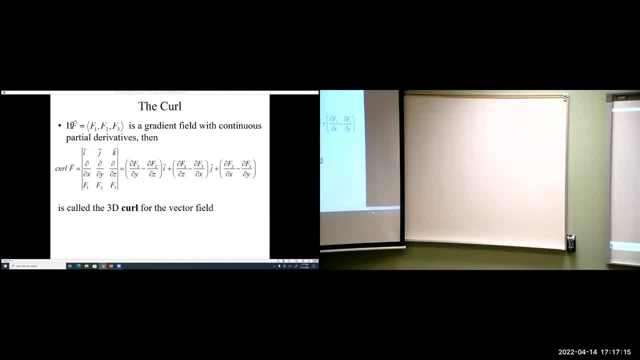 And that just tells us which way it's spinning: clockwise or counterclockwise, Because it's either coming out of the board or into the board. OK, last thing I want to talk about, and then we're going to look at one thing in Calcplot 3D. 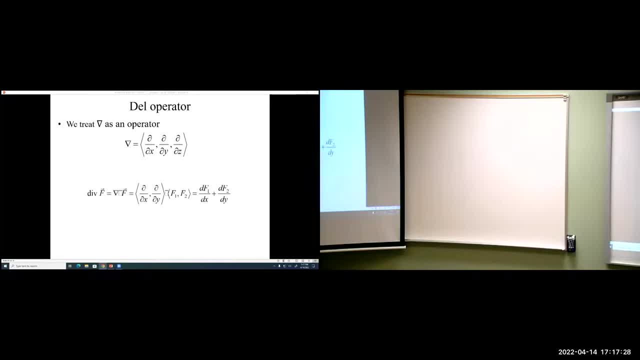 and then I'll let you guys go. The del operator. only because it comes up. there's a symbol on there, That square, the rectangle here should be multiplied. The del operator. remember we saw this in gradient. the del is just telling us. 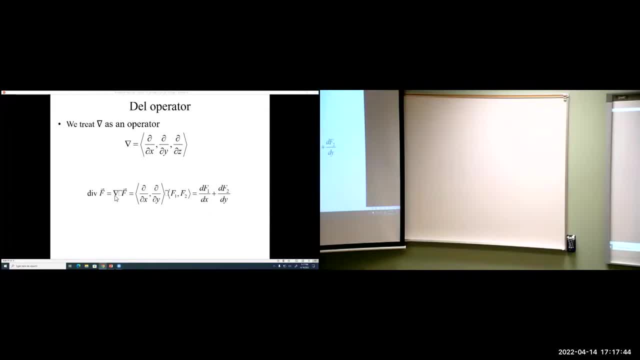 to take the partials. So basically, this is supposed to be dot product, So let me write it up here what it's supposed to say. So when we're looking at divergence of f, that's the del dotted with the vector field f, which means 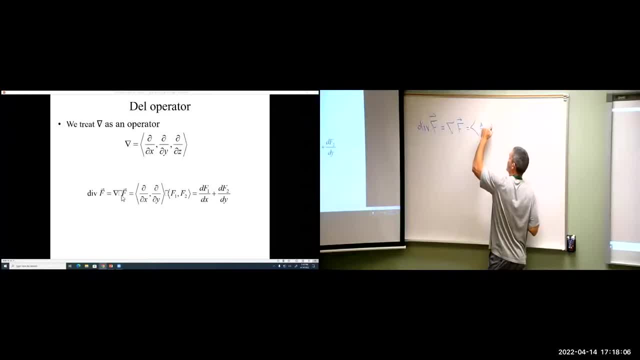 I'm just going to do the 2D. The 3D is just one more component, b, d, y. So this vector field is being dotted with f1, f2.. OK, so we're doing dot product, so that. 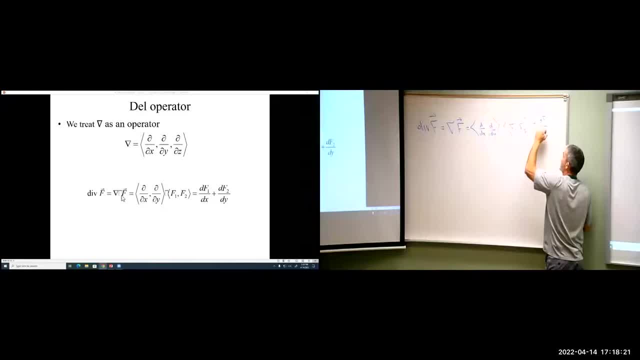 means df1, dx plus df2, d1.. So that's all that's saying. There's nothing crazy going on with the del operator, it's just we've seen it before with gradient. right Now, this was dot product, so that dot is in there. 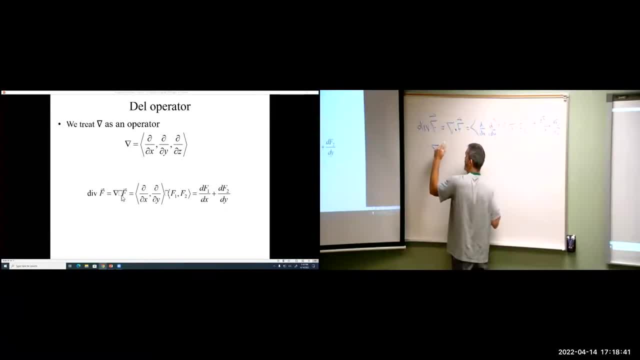 specific. but when we do a gradient of some function, think about what we do right. We do df, dx, df, dy, df, dz. So that's what this triangle- upside-down triangle- it's called del. That's the way it's working in these. 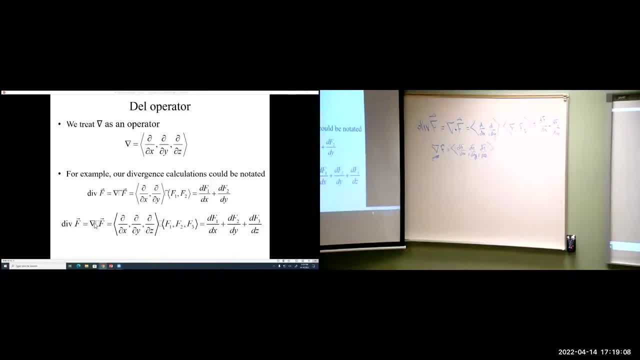 Question in the chat. Sorry, Gabriel. Question in the chat. Someone asked: is the direction? are the directions of the gradient perpendicular to the force field? Are the directions of the gradient? the gradient is the vector field. They're perpendicular to the level curves of the function. 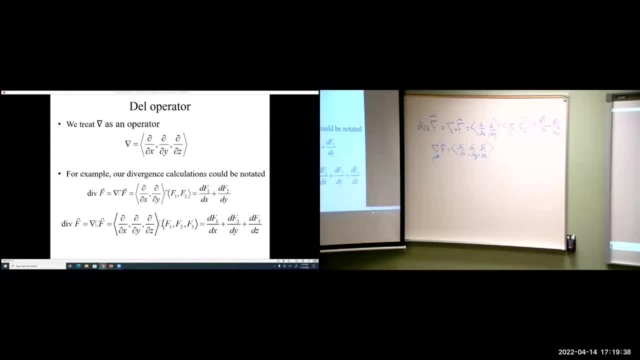 Catherine Hurley. So when we find a gradient field, we've found a vector field. So the only thing that they're perpendicular to are the level curves of the original function. Sorry for missing the question. Didn't have a chat open. My Dot operator is missing on this one too. 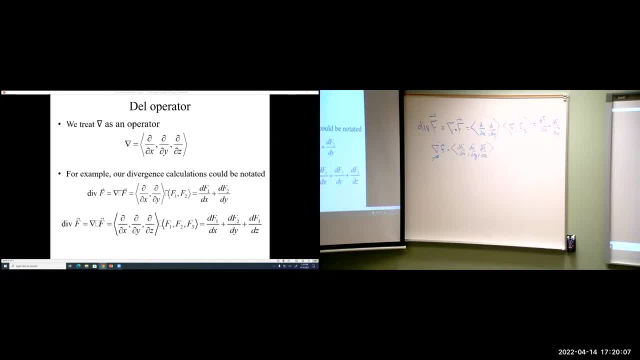 but it's a thumbs down, the same idea. So that's what del is. It's not a major concept, It's just an operator telling us to take the partials of the function or the vector of the vector field. Okay, Let's do one thing that I think is kind of cool, And then we'll go over to the worksheet. 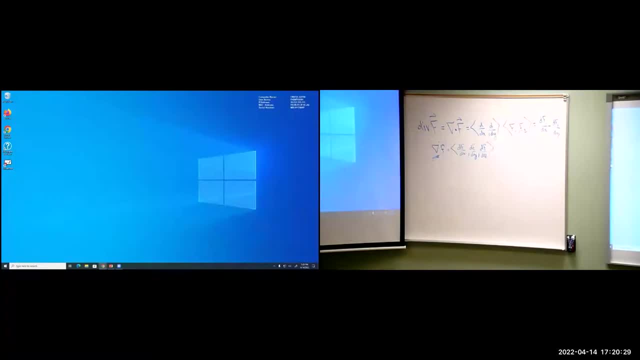 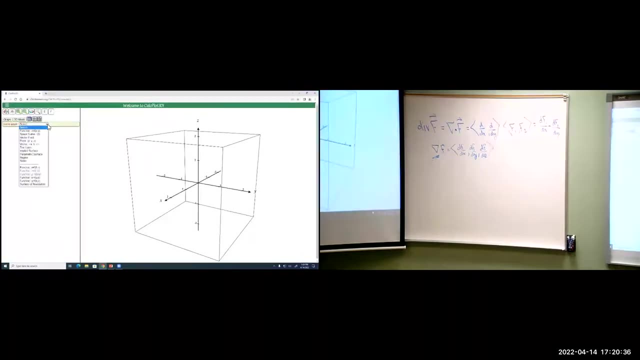 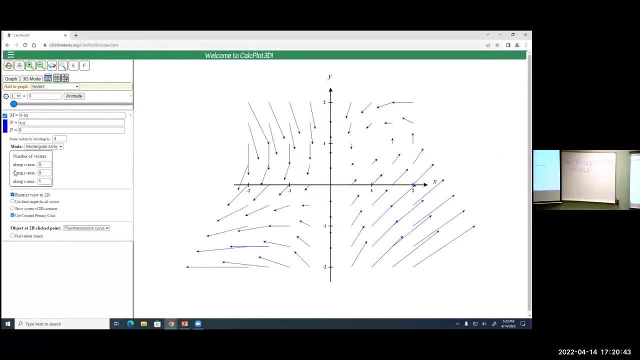 So let's. this is something you guys can play around with. but calc plot 3D, Bring up a vector field. I'm just going to use the one they have in there. It's only a 2D vector field, So let's just restrict it to 2D. 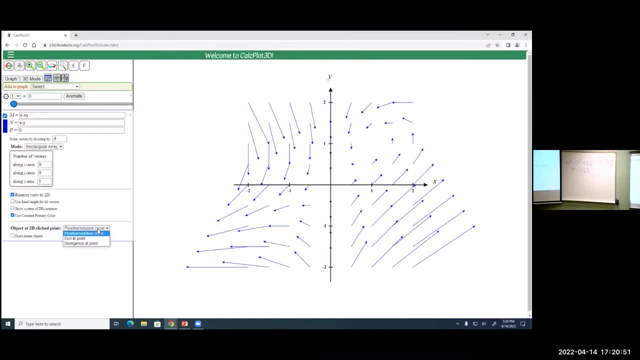 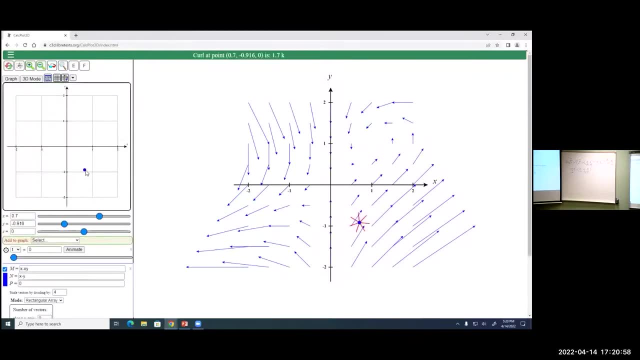 Okay, Now we saw we could do flow line solution, curve. We can also do curl at a point, So let's drop a point in there. That's the curl. That's what's making it rotate. Now watch what happens as we move this point around. Notice how, oh gee, where- the vectors are longer and 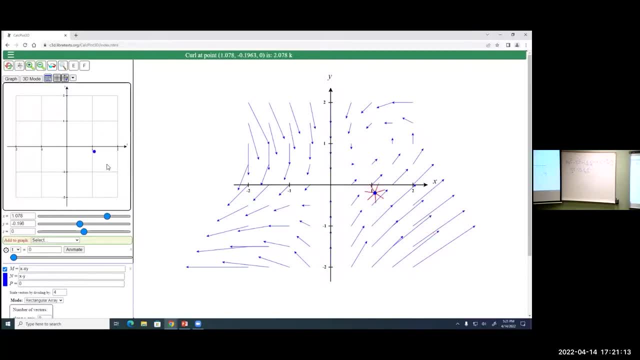 in the same direction, it starts rotating faster. Right We can find different spots And at any of these spots we can calculate the curl, because we know how to do that right. It's that df2 minus dx minus df1 dy. 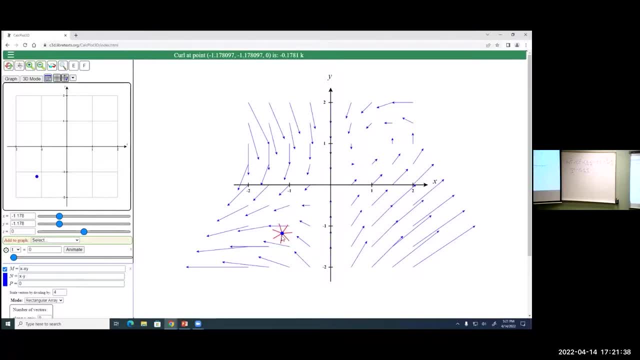 So at any given point we have a curl. Look, there's the curl going in the opposite direction. So that's telling us the curl is negative in this case, because right now we're only looking at a 2D curl. So by all, this is something that we can, that you guys can play around with for the vector. 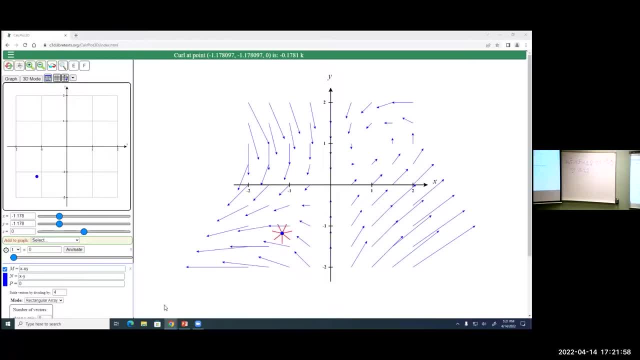 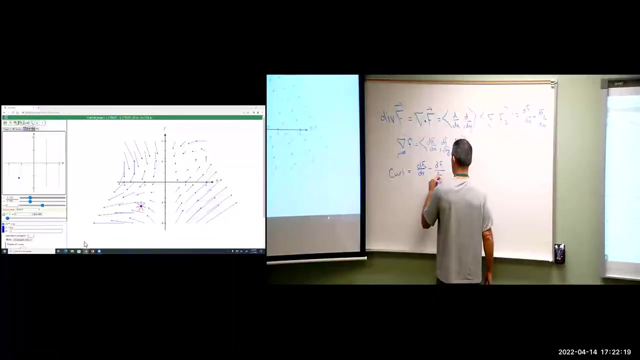 field you're looking at Now. I just did the 2D curl, So now we're looking at a 2D curl. So this is the default one on here, but we can actually calculate the curl for this. So our curl- again we're just doing 2D right now- is df2 dx minus df1 dy, which for our vector. 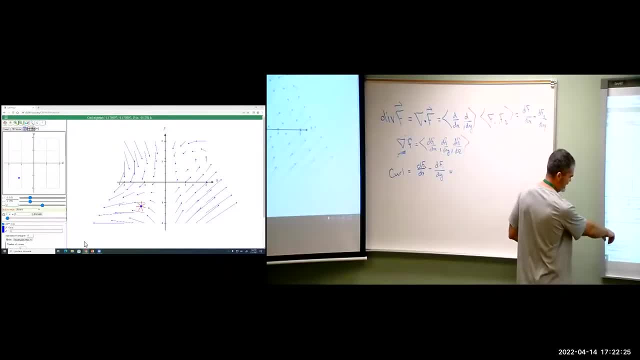 field. if you can't see it, it's m and n. m is f1.. n is f2, so df2, dx. so i'm taking the derivative of n with respect to x, which would just be one, and then df1, dy. so the derivative of this guy with respect to y, well, x with respect to y is zero. 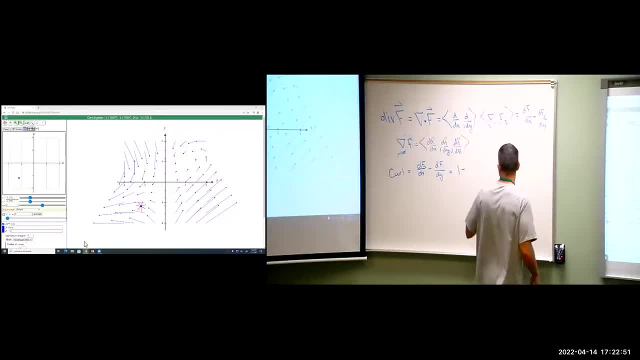 and negative xy with respect to y is negative x. so one minus negative x or one plus x. that will give us the curl at any point. and it makes sense that it varies because we saw that the rotation was different depending on where we were in the vector field. if the rotation had been 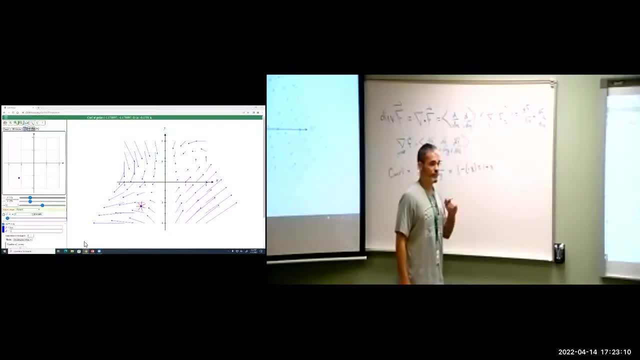 constant. we would have expected this to be constant. the vector. if it would have been zero, we'd expected it to be zero. in fact, let's. here's a vector field. we looked at this one last time- yx. we calculate its curl. well, df2 dx is going to be one, minus df1 dy, which is one. this has a curl of zero. 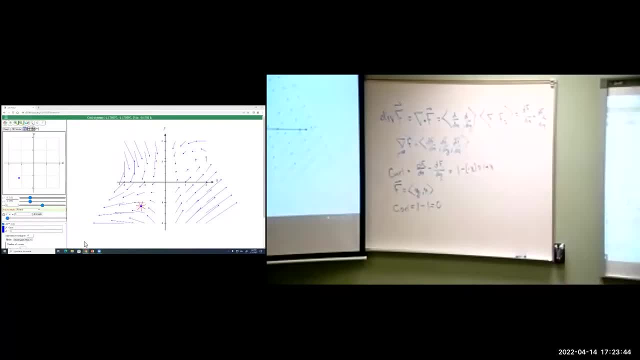 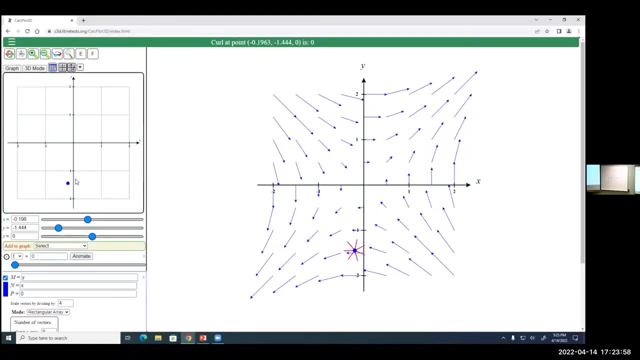 everywhere. that's its general curl. all right, now let's see. so we're going to put in yx now. when i move that point around, no matter where i have it, there's no rotation. that's what you should see in a conservative vector field or a path independent vector field. 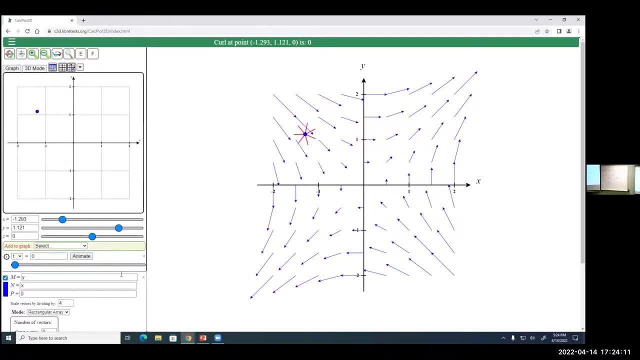 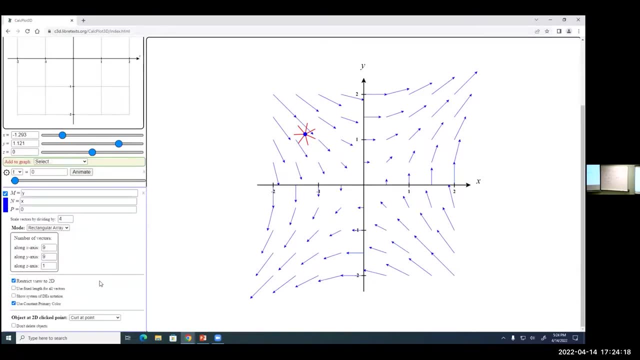 that's what it looks like when our curl is zero, right. so that's something. uh, this is something you guys have access to that you can play around with when you're working on a vector field. it'll work for 3d vector fields too. um, it's uh, i gotta get this out of 3d, okay, so 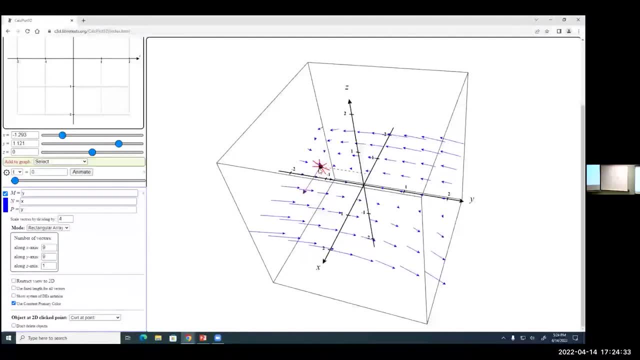 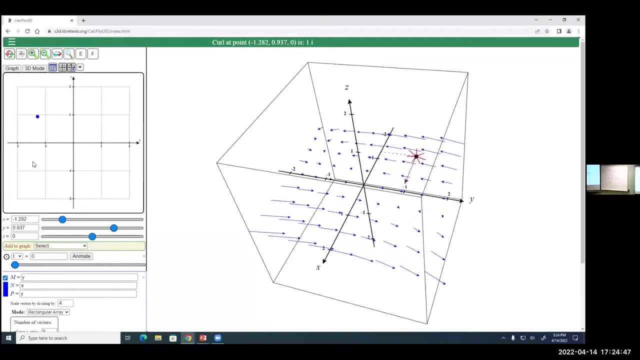 you can see here. it even puts in the vector for us now because we're in 3d. that's that axis of rotation we were talking about and you can move that point around and we can see. depending on where the point is, we have a different rotation. 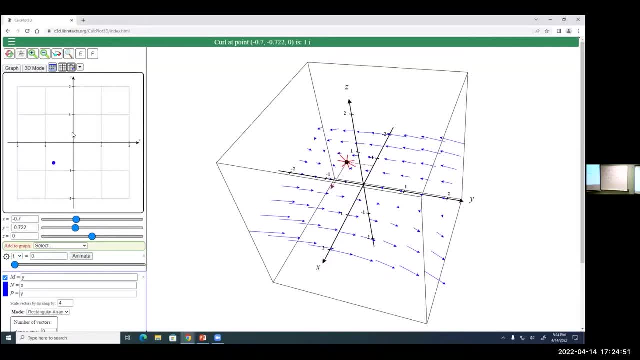 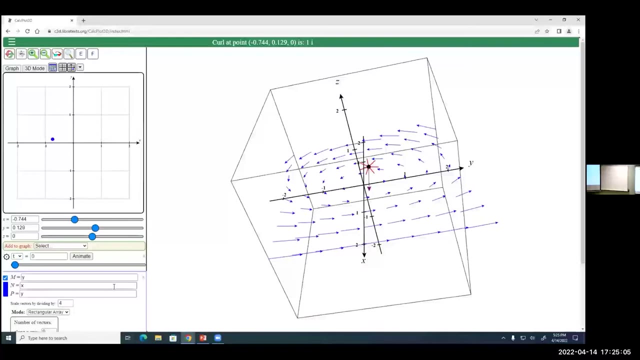 in all of these um, that's rotating the same way, see, which is why i'm going to move that point around. so that's why that purple vector is always pointing in the same direction and we can see it's a three. it is in fact a 3d vector field. 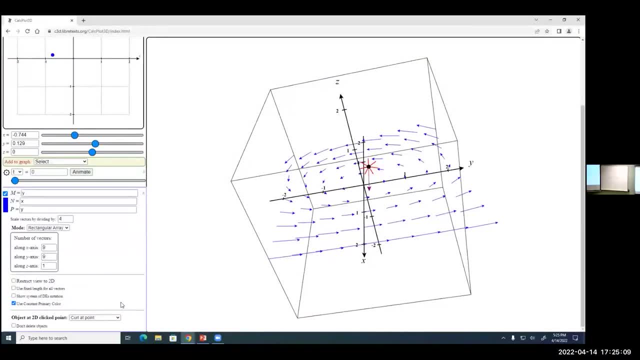 the other thing. again, this is something you guys can play with. you can play with it as you work on the worksheet or you can play with it on the homework, just to kind of start to get a visual of what the heck is going on with this curl and divergence. 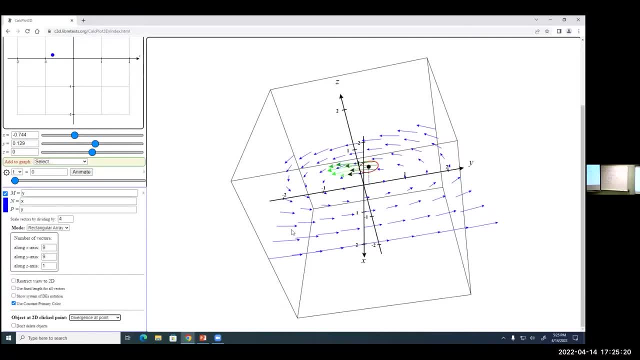 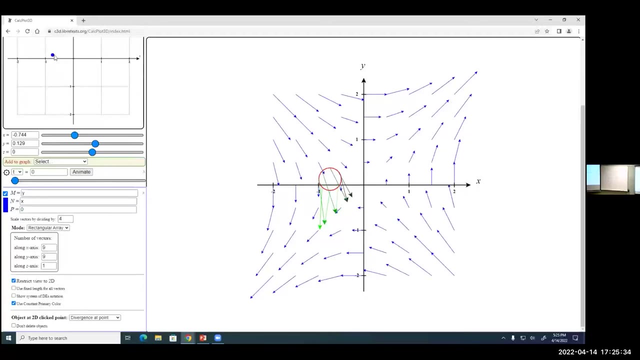 they can do divergence at a point- remember it's the amount going in- or to a point. so the point is that let's, let's go, let's start off in just 2d here, let's get, let's take that out of here for right now. okay. so here's our divergence and now the 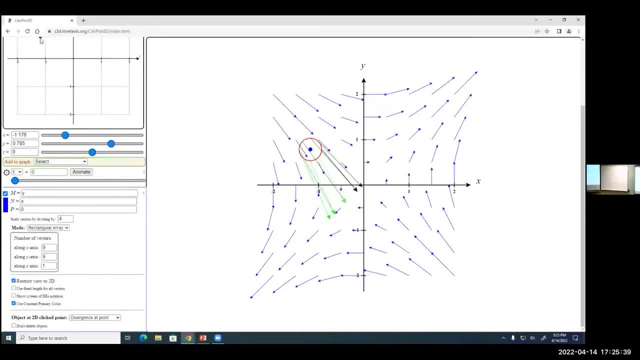 way this works is: you know, we've got the circle, this point. here is the point where we're measuring the divergence. the circle is kind of saying: okay, well, what's going in towards the point, what's going out towards the point? so these ones that lie inside the circle, 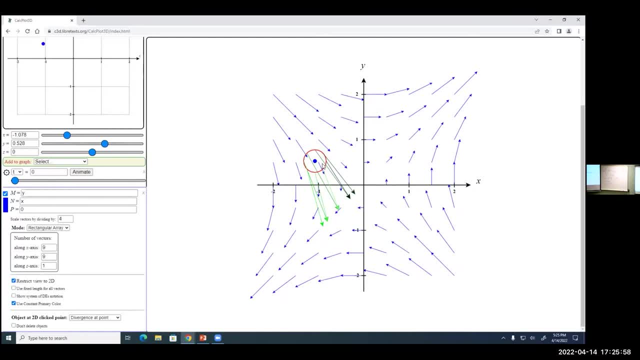 are sink are sinks. they're being attracted towards the point. these ones that are starting outside the circle and being repelled away, those are representing a source at the point. so let's go to a very nice, easy point. let's just do one more, okay, all right, so we see something. 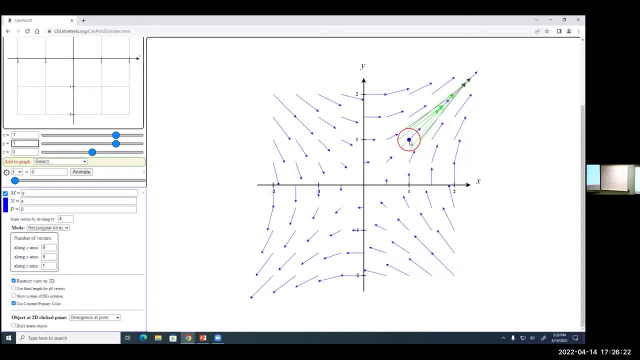 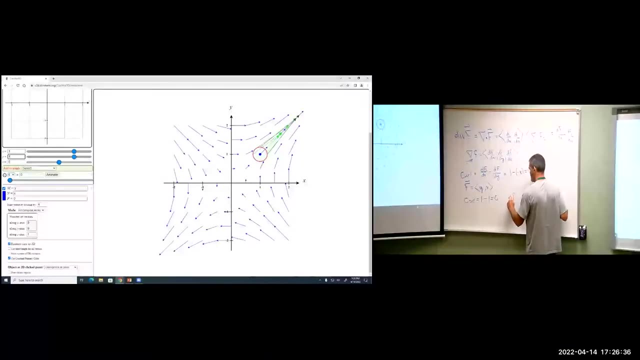 like this and we want to know: okay, well geez, is that a source or a sink, or is it neutral there? remember, we can calculate this. so now i'm doing it for this, this vector field here at. i didn't go back to the original um, so the divergence, oops, sorry, the divergence of f. 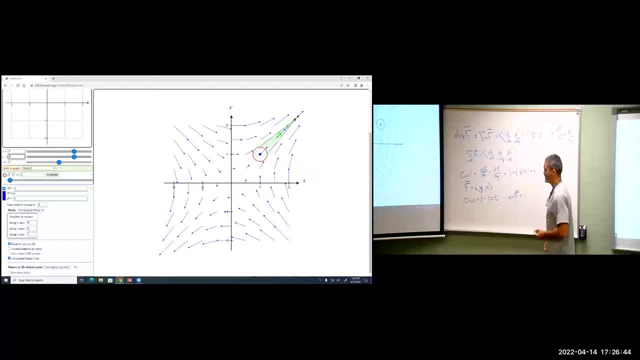 it just comes from adding up the partials. well, the derivative of y with respect to x- oops right, it's a scalar- is zero. actually, it's great derivative with respect to x of y, plus the derivative with respect to y of x is zero. so that tells us that at any point in this gradient field, these things are in balance. 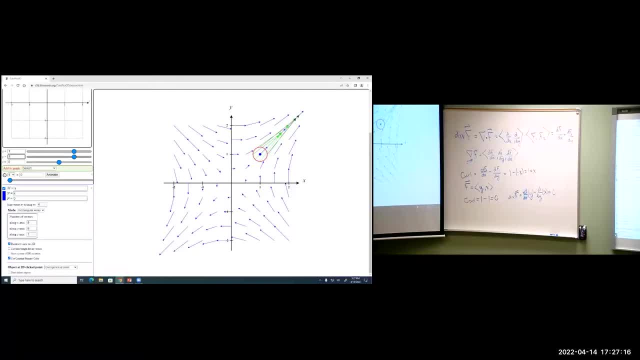 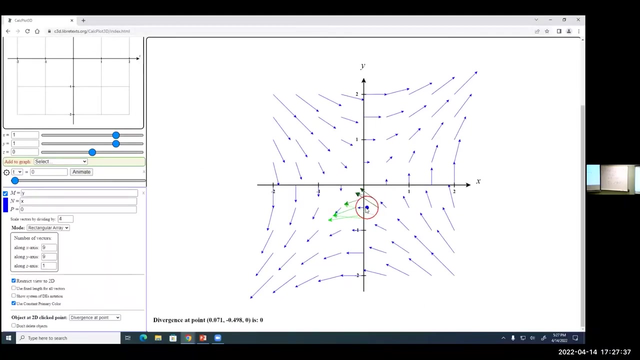 there is as much going in as there is coming out for this particular gradient field. okay, and what we would do is we look at two things: we look at how many of them are going into the circle, but also the magnitude of them going into the circle, and you can see right here, right here at the bottom, it's calculating the divergence for us.